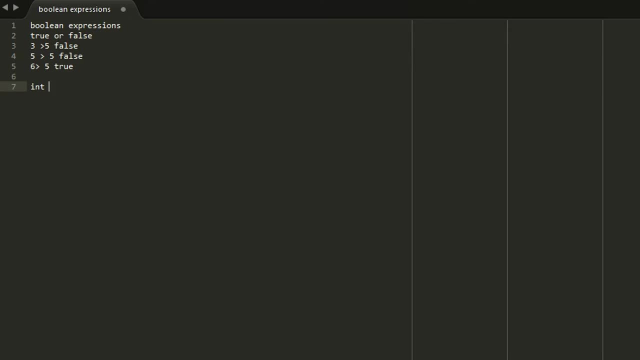 also use variables. So if you said int x equals three, x is less than five, then that would be false. So those are some basic examples. There are also a couple of operators that you can use, but the basic ones you'll usually use are less than greater than. 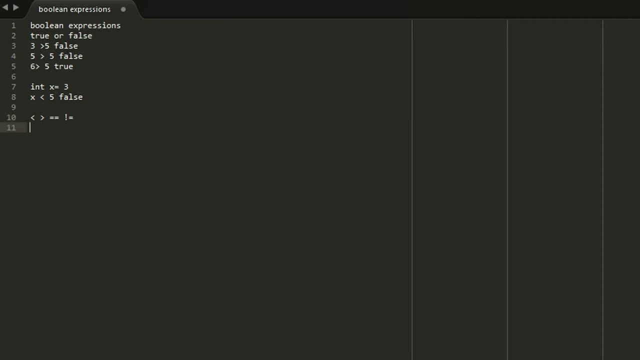 equals, not equals, and there's a bunch for strings and stuff as well. The basic boolean operations are and, and, or So and is basically what you see on the screen. So true and true is true, True and false is false, because nothing can be both true and false And false and false is. 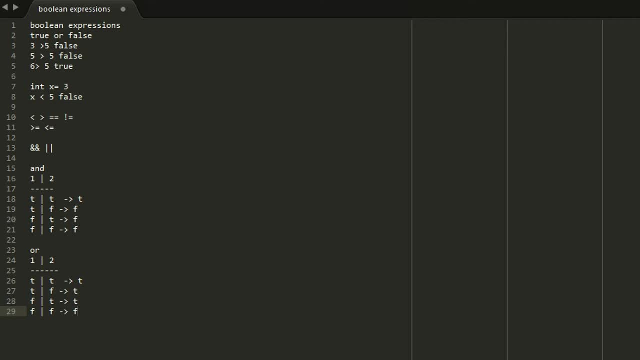 false. Ors, however, are similar but not the same. So true or true is true, False or false is false. But true or false is true because it has to be either true or false. There's nothing in between. So what you see on screen, 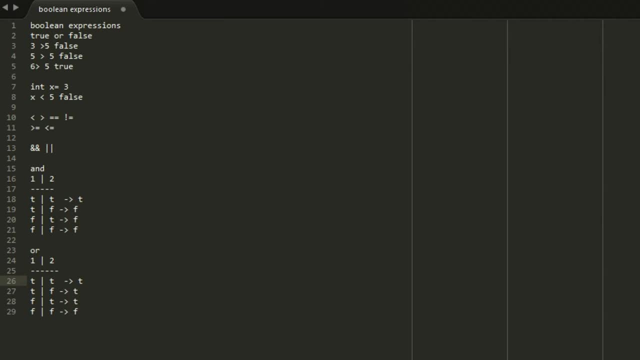 pretty important Memorize and continue to the next part. Alright, guys, so now we're going to cover the very basic conditional statements, And the statements I'm going to cover today are if, ternary operators- which aren't really statements but similar to ifs- and switch statements. Alright, 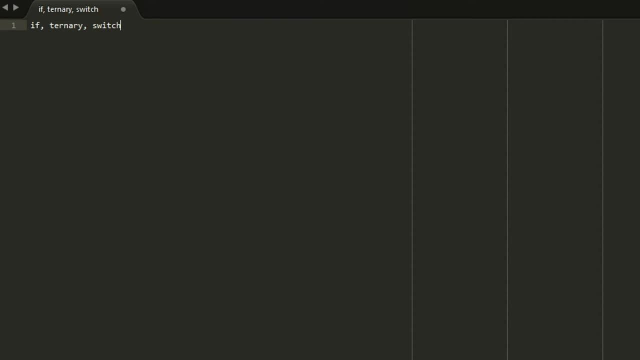 so first we're gonna start with the if statement. Now an if can be read in English, so it's pretty easy to understand. So let's say, for example, you have variable x and if x is less than three, you want to print out the word hello. In that case we would write something like this: 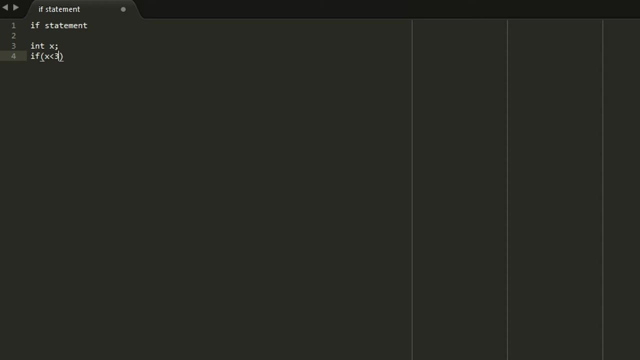 If X less than three: curly braces, console dot log hello, And then that would print out the word hello if, and only if, x is less than three. If you wanted to print out goodbye if x is greater than 10,, you could add a little bit to that if statement, which would be: if x is less than three. 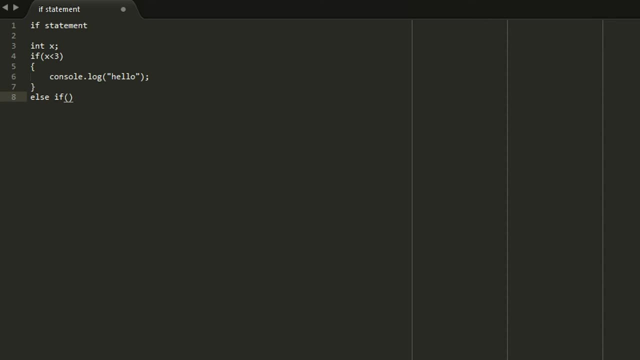 console log hello Else. if x is greater than 10, print bye or console log bye. So that's how that works. And the final thing that you can tack on to an if else statement is just a plain else, which is a catch-all. So if you wanted to print out the same stuff, like we had before the hi and 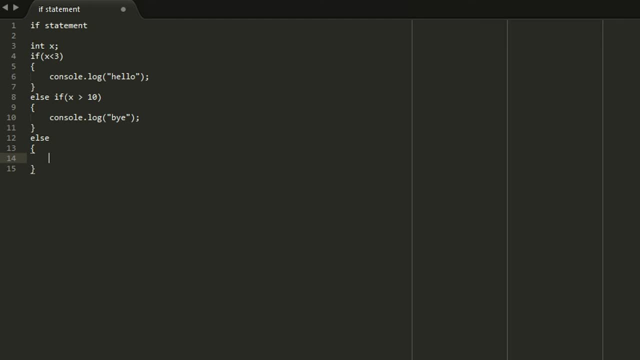 the bye, and then in between you just wanted to print out something else, I don't know: abc. Then you could have what you see on screen, which is: if x less than three, print hi, else if x greater than 10, print bye, else print abc. And then that would accomplish that. Next we're going 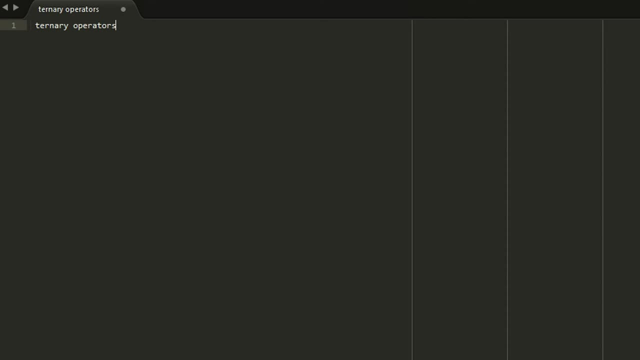 to cover ternary operators, which are pretty much like if statements, but you can use them in line, which is pretty cool. So if you were making a string and you wanted to use a variable and you wanted to say something like: x is blank five if it's greater than five or less than five, then you could do something like: 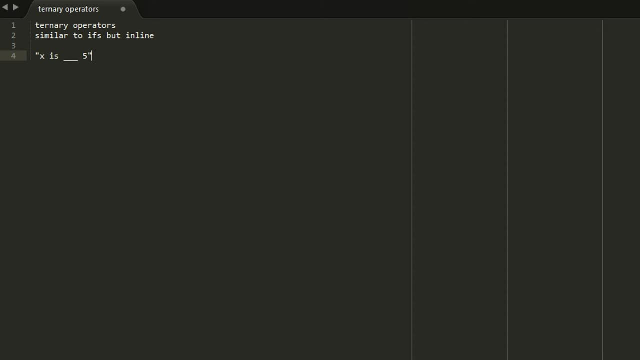 this. So you would say x less than five question mark And if that's true, then you would say less than, because I would say x is less than five. Or you could say greater than or equals to for the other statement, which would come after a colon, like you see on the screen. 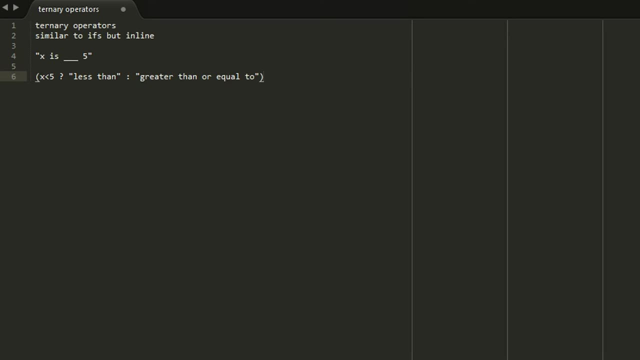 So it's basically can be read the same as an if statement, but the syntax is a little different. Next, we're going to go ahead and cover switch statements, which the switch statement. it's pretty similar to an if else kind of deal, except for it's more organized in my opinion. So you 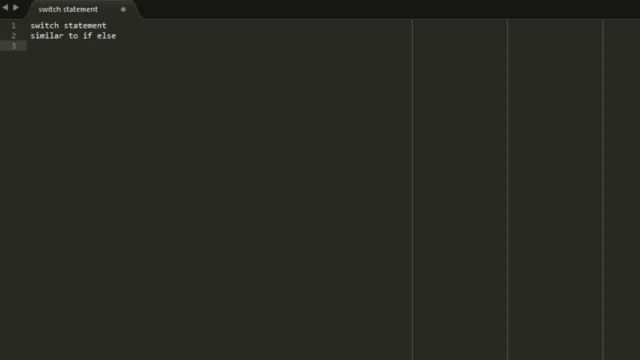 wouldn't be able to do as much with it because it's just, it's not separated in blocks and it's prone to having issues. So what you're going to do is say switch and then the variable that you're trying to compare values. 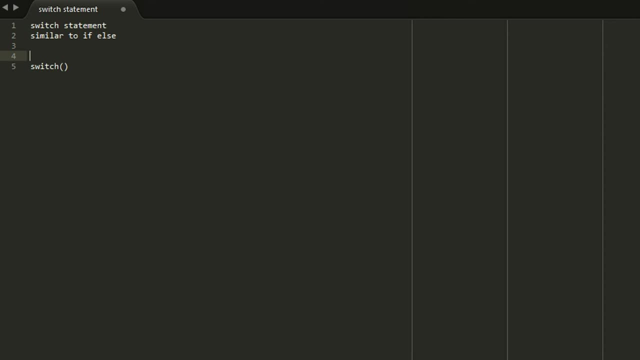 with. like if we want to do different things with the variable x, if we want to print out numbers in word form, but only if x is equal to one, two or three, then you can say: switch x, case one, console, dot, log one, break. so you need to do the break or else it's going to run through all of the commands. 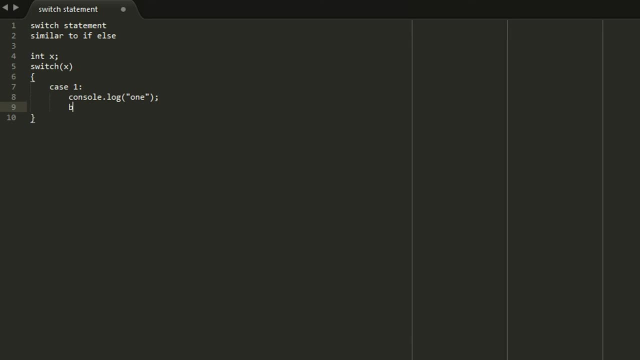 in a row And then we would have case two, console log, the word two, so on and so forth. This also has something similar to else, where you can actually type the word default and then that will catch everything. So, like I mentioned before, it's really important that you guys use the keyword break, or else it. 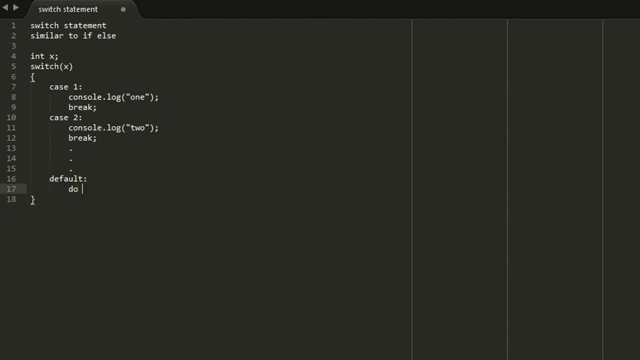 will run through all of them and you'll have a really frustrating bug that you have to track down. All right, so that pretty much covers conditionals. Next, I'm going to do a brief overview of loops. If this isn't clear enough, I can give it a dedicated video, since loops are a little bit confusing. but 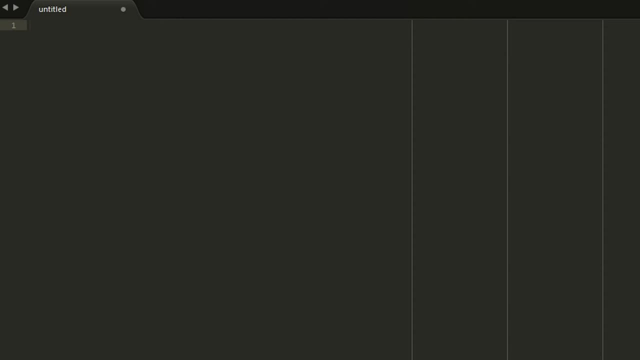 the three types of loops I'm going to cover today are for, while and for-each. Now we'll start with for, and this is something. there's a bunch of different syntax, so I'm just going to show you the most basic. You can start by making, say, an integer is probably the easiest example. 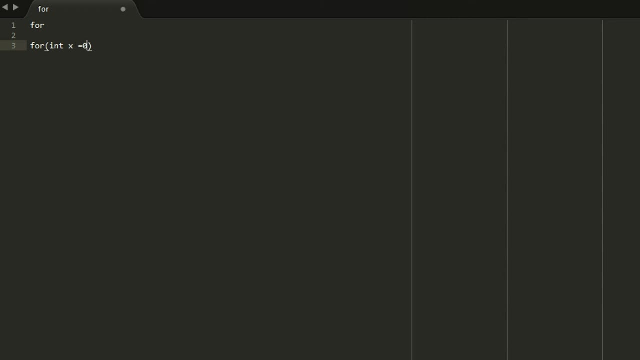 So you say: for int, x equals 0, so that initializes x to be 0. And then the next part after the semicolon is the statement that needs to be true to continue, which is: x is less than 5.. So, while x is less than 5, we'll run this loop. And the next part is what: 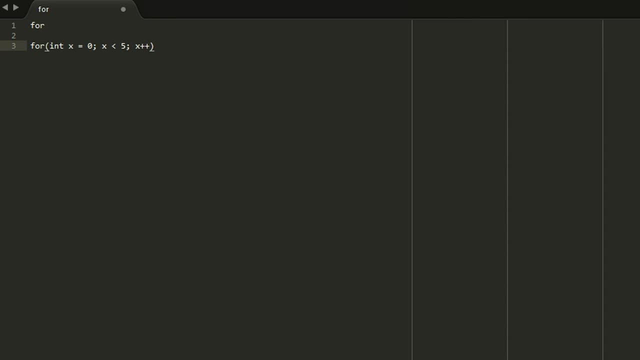 you're going to do after the loop is done. So we will do x++, which is basically the same thing as x plus 1.. So inside this loop you can just see that we're printing out the value of x. So this would print out 0,, 1,, 2,, 3,, 4.. Because 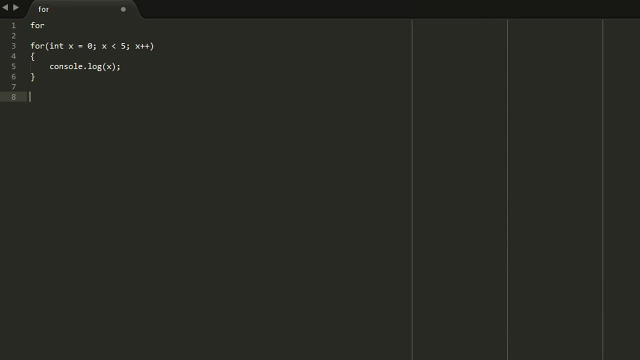 when you first go through, it's going to be equal to 0.. You print out the value, You add 1.. Now the value is going to be 1.. You print out the value, You add 1.. It's going to be 2.. And then, eventually, it's going to get to 4.. You're going to add 1.. 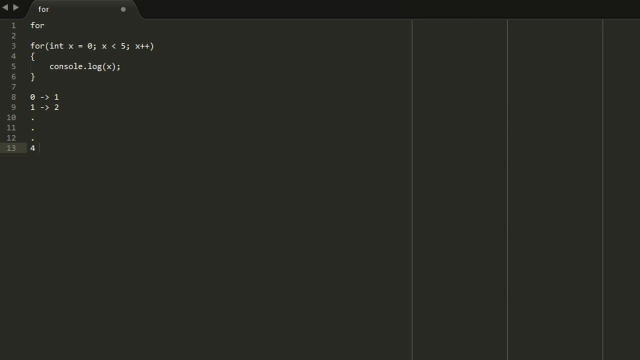 And 5 is not less than 5, so it will stop. So that's the basic of 4 loops. While loops are very similar to x, they're not always the same. They're not always the same, They're very similar to 4 loops, except it would only be the middle part. So you're. 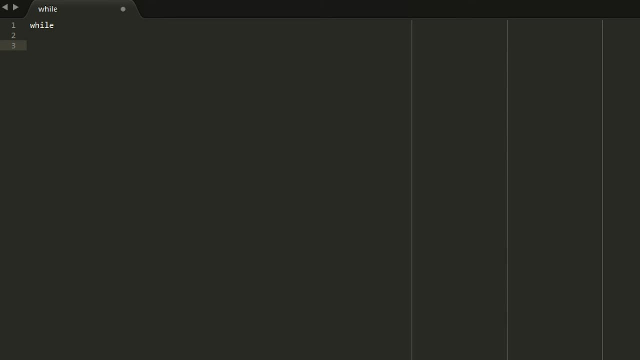 able to do while, true, and that would be an infinite loop, which is not great, But sometimes you want to do that because you don't know how much input is being put in, or other situations where it's appropriate. But a lot of the time while loops are used kind of like 4 loops. 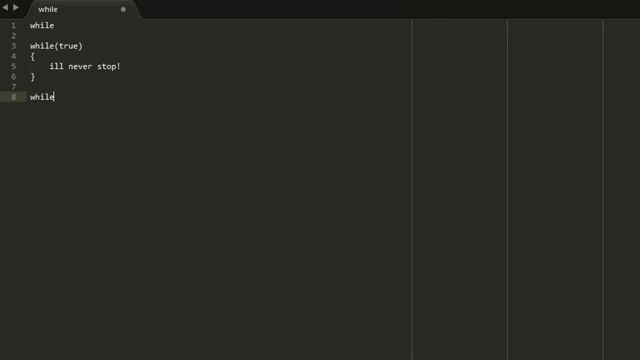 So you can initialize the variable above and say: int x equals 0. And then you'll have while 0 equals less than 5. And then you'll have consolelog, And then at the bottom, instead of not putting anything, you'll put x++, And that's the same thing as the for loop. 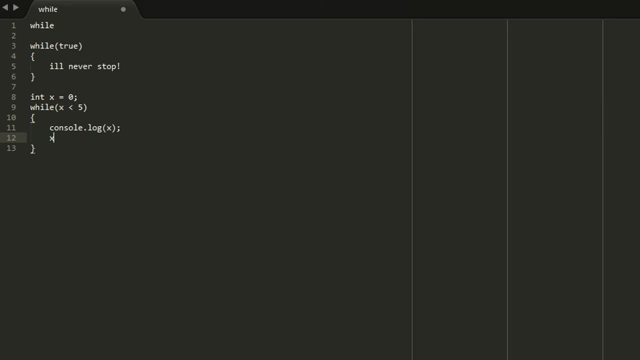 You can also break out of the while loop and the keyword literally is break. So if the expression was: while x is less than 5, but for some reason you actually wanted to break out when it was 3,, which wouldn't really make sense. But let's just pretend that's. what you want, So you can actually keep putting this more than 1, even if it's flip, And this way you can get 4 loops. So it's going to become u 2, and if you forget all the loops here, 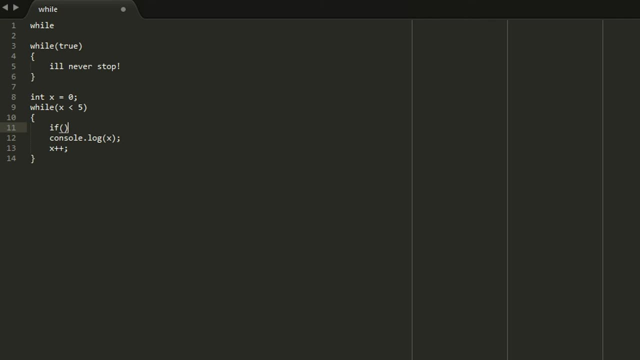 you can get 1 loop in the first loop And you can use that option to compute the value for the than 5, and then you can say: if x equals equals 3, which means if x is 3, break. So when it hits 3 it'll break. else. consolelog: x, x++. 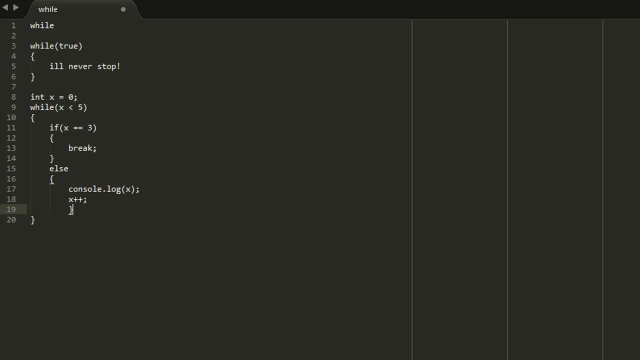 Now that will effectively print out 0,, 1,, 2, but it won't print out 3, because that's what you specified in that if statement in the while loop. So that's the basics of while loops, And then finally we have a for each loop. 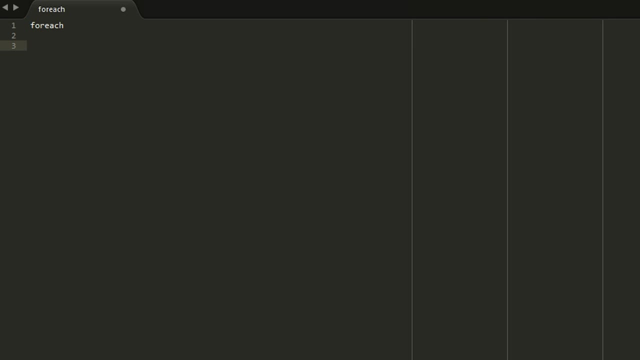 Now, not all languages have it, but this is a pretty nifty loop. So I believe I covered arrays in a previous tutorial and basically a for each loop will parse through an array. So okay, say we have this array And it's obviously just an int array with 1..